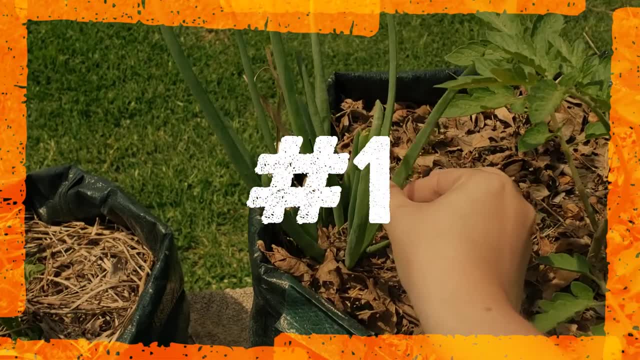 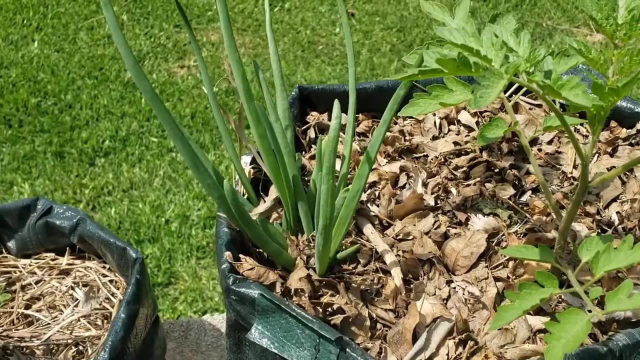 Plant number one. it's kind of squishy but it feels hollow, not like a succulent, and it's branching out very large. Hmm, I wonder what that one could be Over here we have plant number two, and if you look at these, 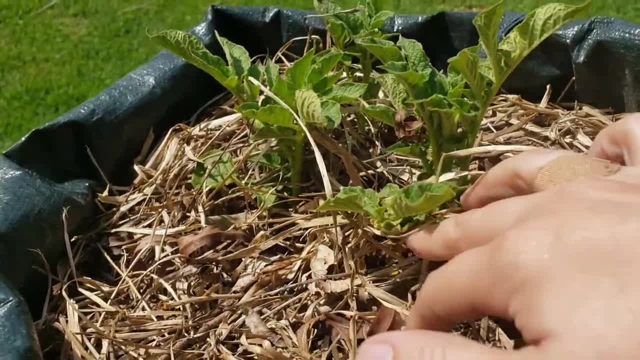 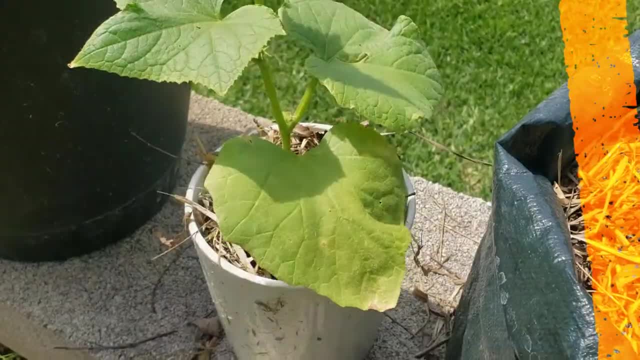 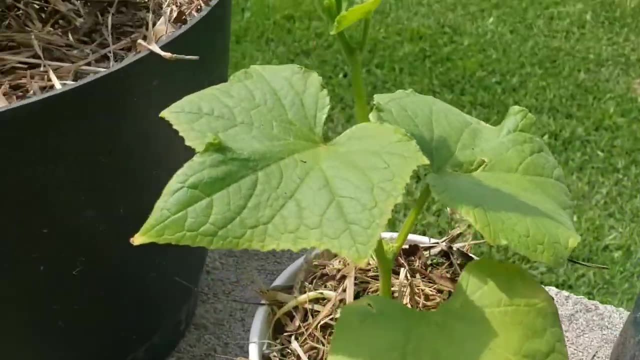 leaves. they're growing very low to the ground and the leaves are really wrinkled up and very small. This is plant number three. These leaves are gigantic. They're about the size of the palm of my hand and then up at the top right here. 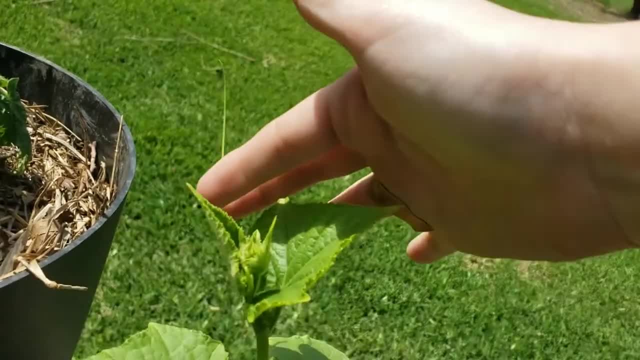 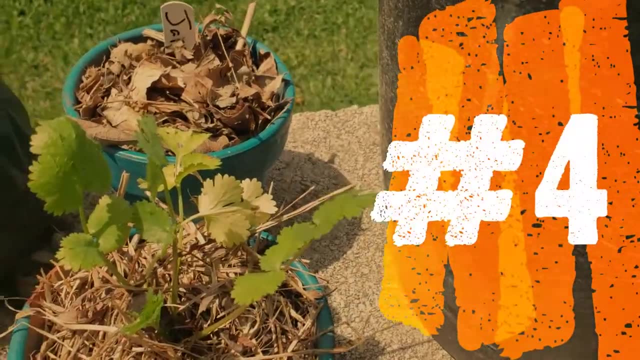 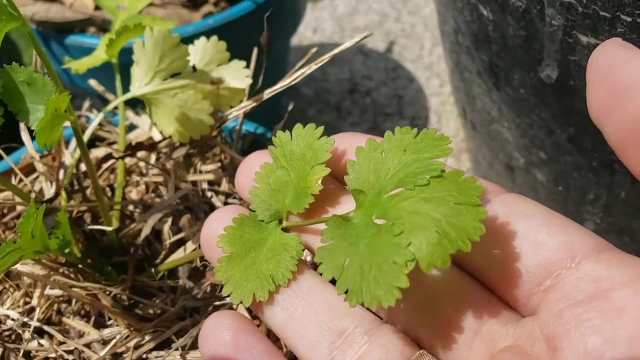 we have a little thigmatropism branch that will curl up around anything that touches. Look at these gigantic leaves. Hi guys, this is plant number four. I will give you a hint: this is one that a lot of people eat. so compared to the size of 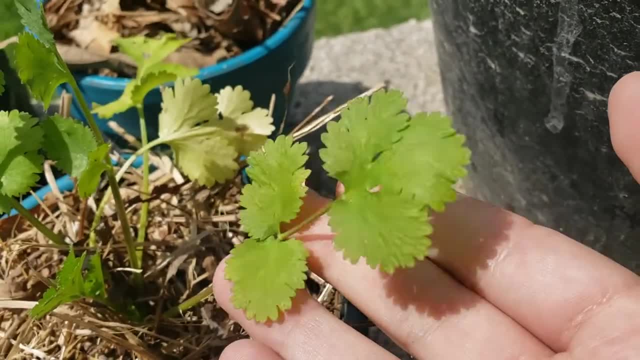 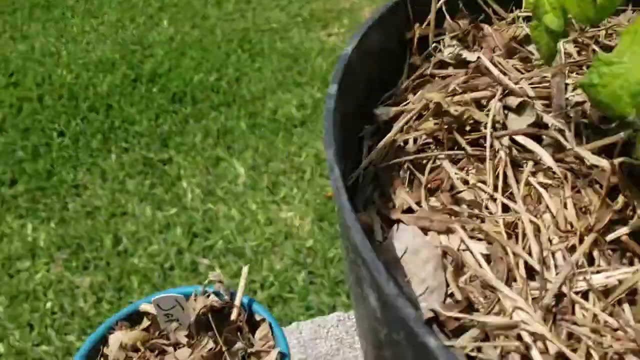 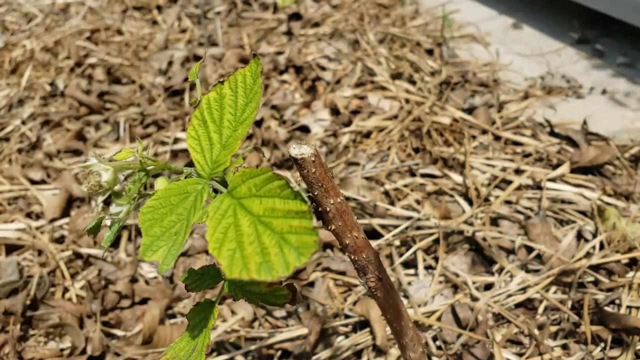 my hand. the leaves are pretty small, very different shape than what we saw from plant number three, which was this guy with the huge leaves over here. So plant number four. Hi guys, we are looking at plant number five and this is probably four, my favorite color leaf. I don't know if you can get the. 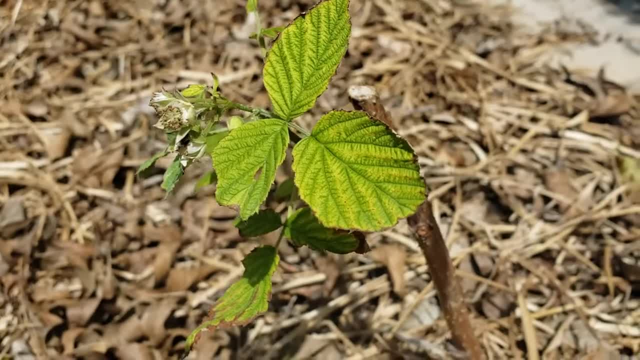 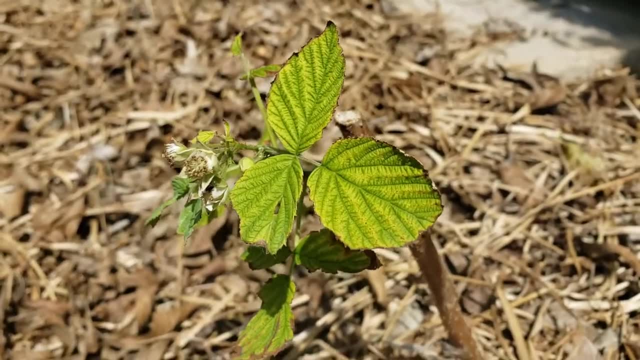 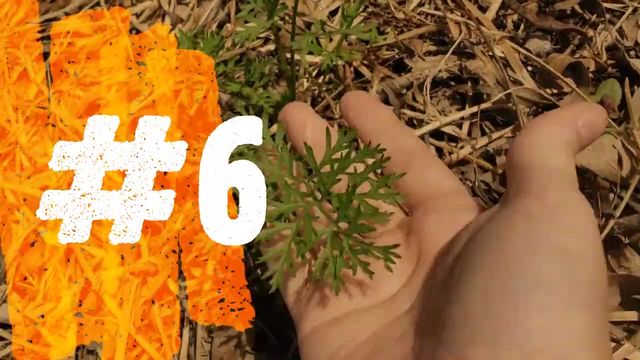 amazingness of these colors in the video, but they are streaked with dark green in the middle and they're pretty small. Oh, I'll have that fall over. It's just like right in the middle of the garden. All right, here's leaf number six. These are very different in shape from any of 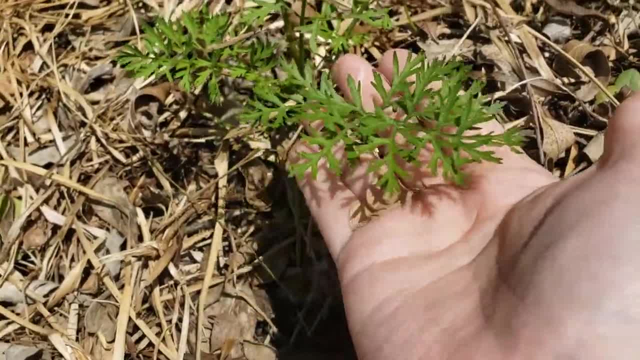 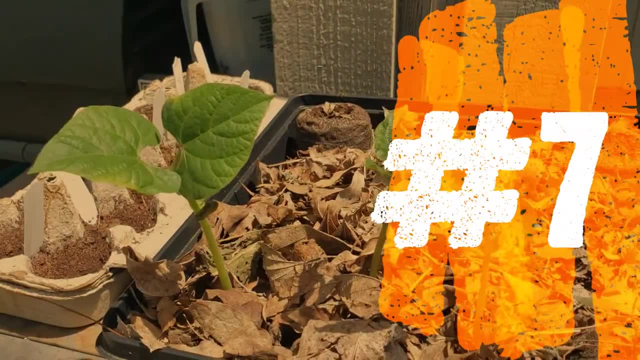 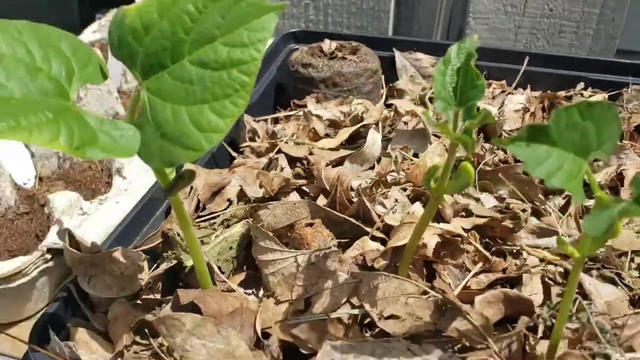 the ones that we've seen before Growing pretty close to the ground here. This is number six. All right over here we have plant number seven. I actually have three samples of this one at different stages of its life. So if you look at these, these are very. 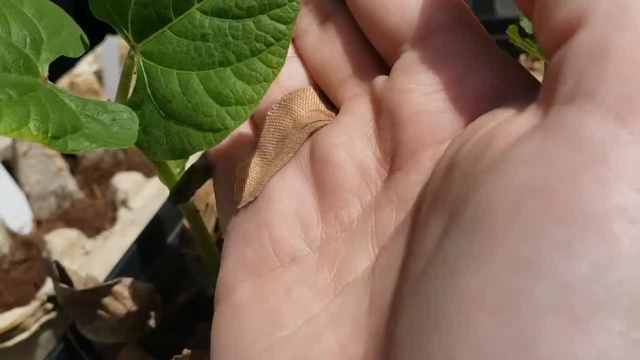 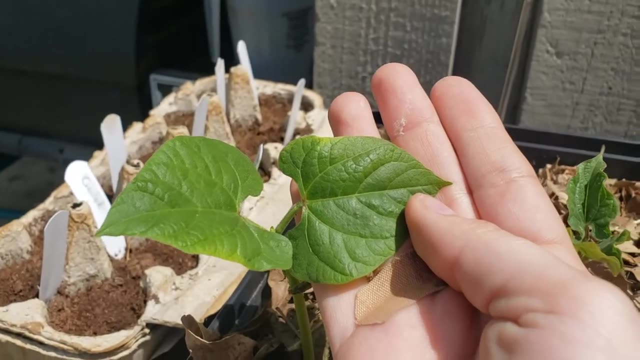 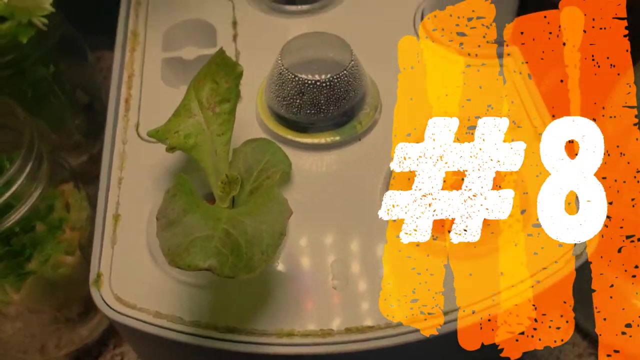 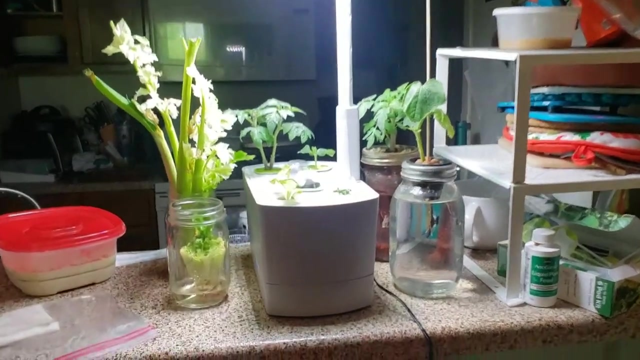 tall in comparison to their size and the leaves are medium sized. I'd say This is plant number seven. All right, taking you guys to a little different location now. This is my indoor system, So it is a hydroponic. If you look inside here it is full of water and fertilizer.